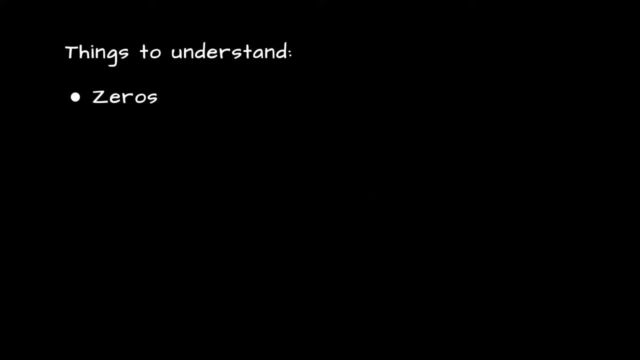 rational expression. Now, if someone were to just hand you a rational function and ask you to interpret it, you might be at a bit of a loss. So what we're going to try to do is be clear about some key things that we can understand about any rational function that someone throws our way. 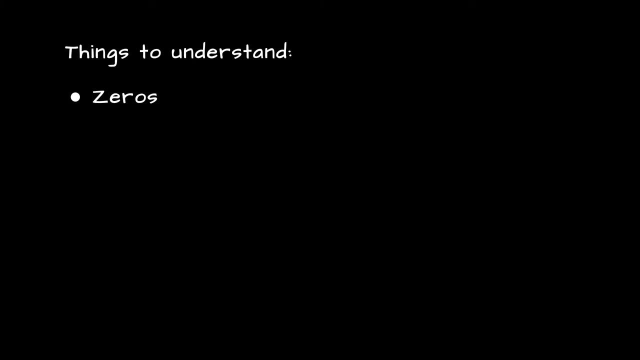 One of those things are the zeros of a rational function. right, As with almost any function in mathematics, we can't understand when it's equal to zero. We would also like to understand, as with polynomials, the asymptotic behavior of a rational function, And there are actually two. 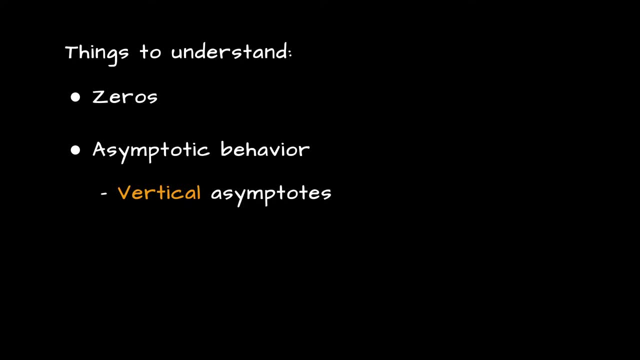 key questions to be aware of. One of them has to do with so-called vertical asymptotes of the rational function, And the other question is to describe the so-called horizontal asymptotes of the rational function. Okay, so so far those are just words on the screen Shown. here is the 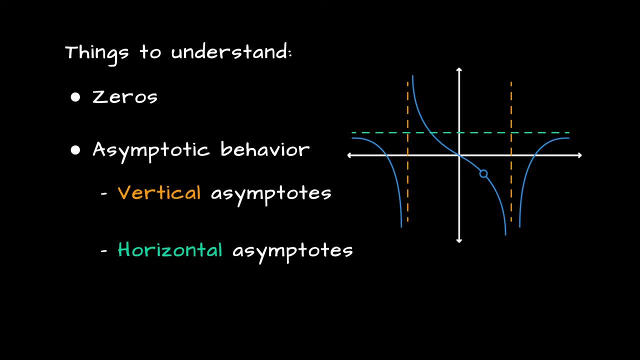 graph of what an asymptotic behavior is, And the other question is to describe the so-called actual rational function may look like. Okay, so the blue curve here represents the graph of an actual rational function. Let's see how different features of the graph relate to the words that we 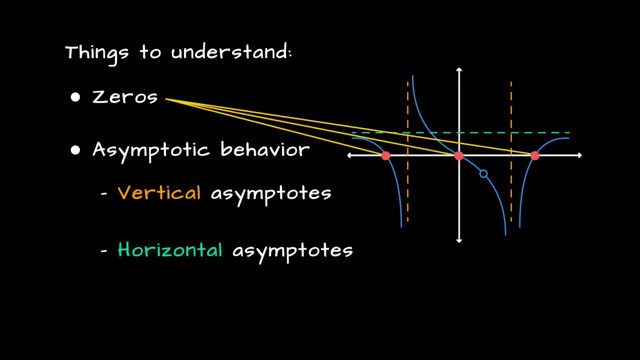 just put on the screen. The zeros, of course, are the places where the graph of the function intersects the x-axis right. They're the three dots shown in the picture. The vertical asymptotes of the rational function are the vertical dashed lines shown in the picture, And they basically 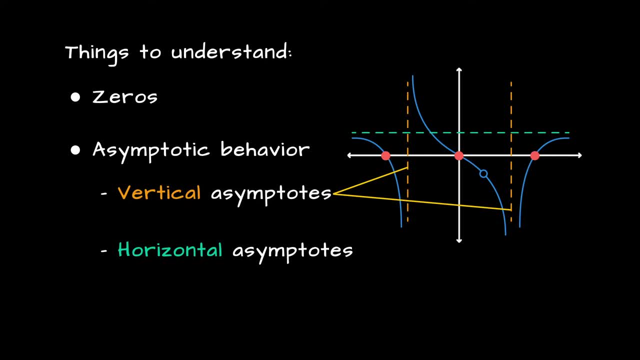 represent values at which the rational function blows up and goes to either positive or negative infinity when that particular value is approached. The horizontal asymptote, on the other hand, is the green dashed horizontal line shown in the image, And it represents a value that the 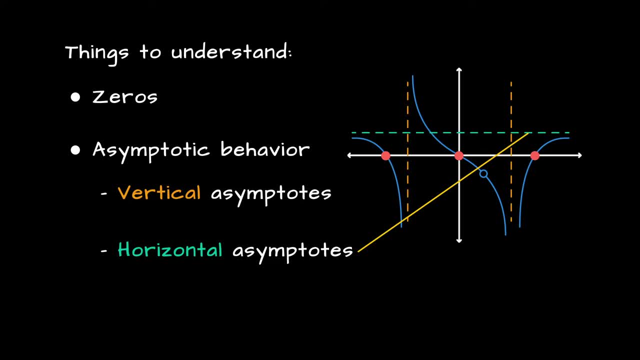 rational function approaches for very large values of x If we go in either the positive or, in this case, in the negative direction. And finally, there's one other feature that we didn't have on our original list, and that's the so-called removable singularity of the rational. 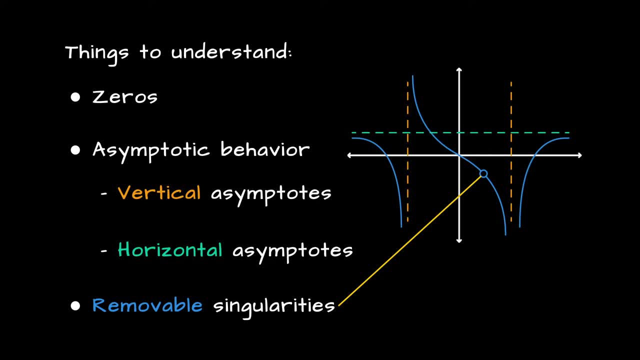 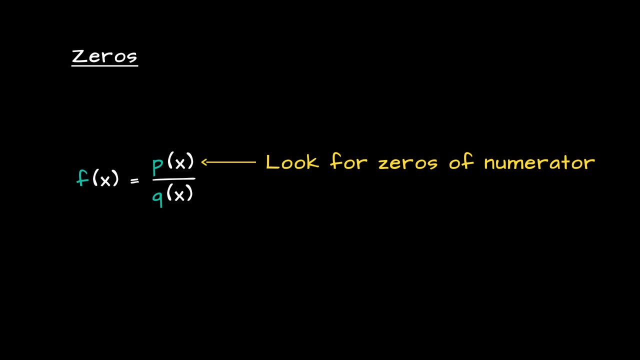 function, And it corresponds, in our picture, to this sort of hole that we've drawn in the graph. Removable singularity is a point at which a rational function is not defined, but where it does not have a vertical asymptote. Now, how can we determine those? 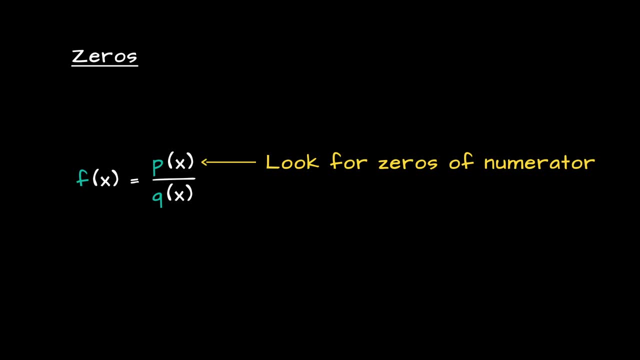 characteristics using algebra alone. What if someone only tells us that our rational function is presented as the ratio of a polynomial p of x and q of x? Well, it turns out that the zeros of the rational function will basically correspond to zeros of the numerator, to zeros of p of x. 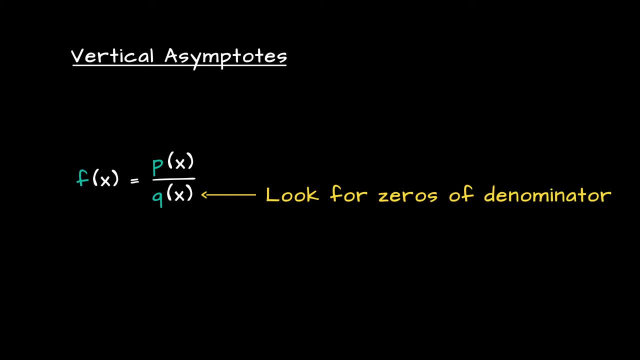 And it turns out that the vertical asymptotes will basically correspond to zeros of the denominator q of x. To understand the horizontal asymptote of a rational function, what we'll want to do is study the degrees of the polynomials in the numerator and denominator and how they relate to one another, And finally to understand. 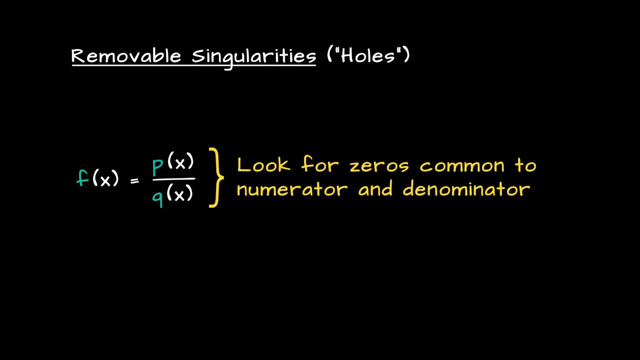 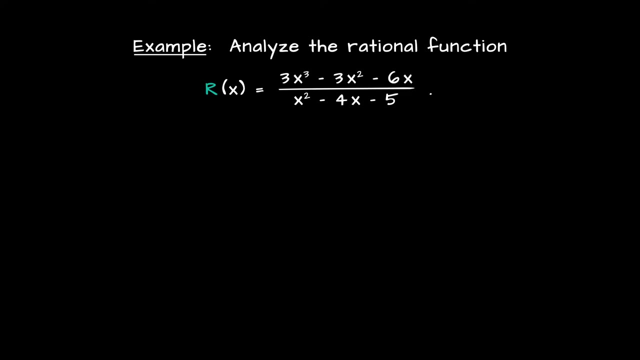 the removable singularities or the holds in the graph of a rational function. we'll want to take a look at zeros that are common to both p of x and q of x. That's the basic idea, All right. so let's try to make all of this more concrete by considering a particular 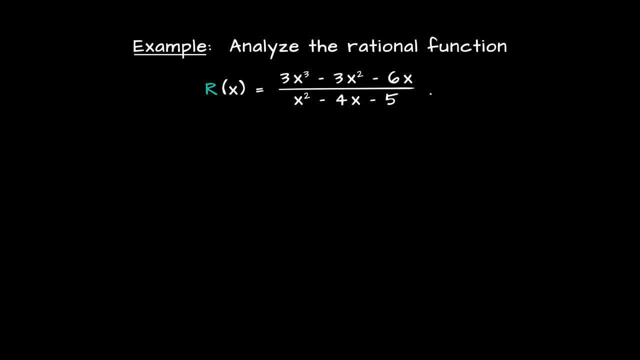 example, We're going to try to analyze the rational function r of x, shown on the screen here, And that means we're going to try to understand its zeros and its asymptotic behavior, meaning its vertical and horizontal asymptotes, and also see if it has any removable singularities. 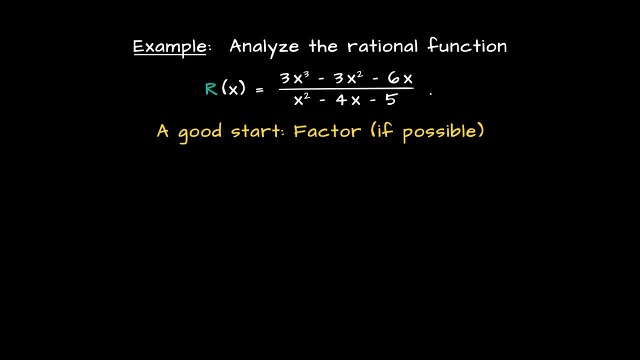 Now a good first step whenever you're working with rational functions is to factor as much as you can. So try to factor both the numerator and denominator of the function. That will make analysis easier. So notice first of all that we can factor a 3x out of the numerator. 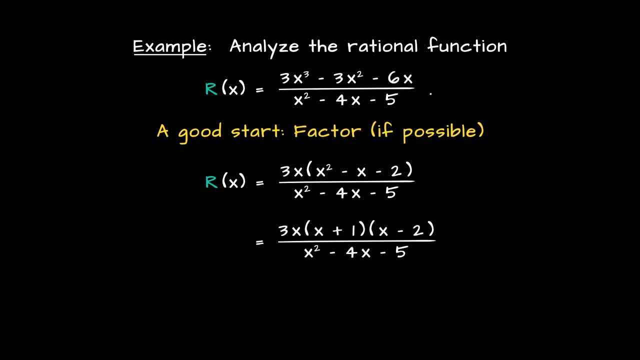 Then the remaining quadratic term in the numerator factors as x plus 1 times x minus 2.. And finally, notice that the denominator factors as x plus 1 times x minus 5.. All right, so here's our rational function in factored form. And one thing we notice pretty. 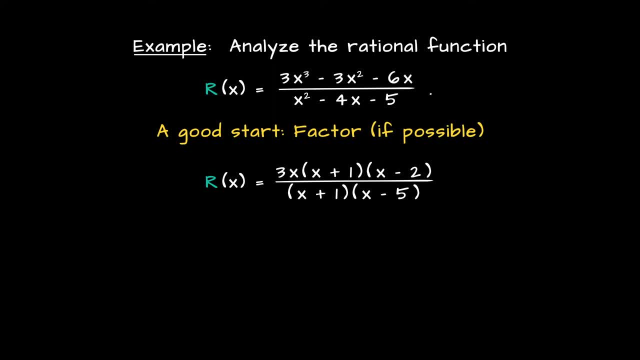 quickly is that there is a factor, namely x plus 1, that is common to both the numerator and denominator. On the one hand, that factor cancels out. But be careful, because the rational function is not defined at x equals negative 1,. 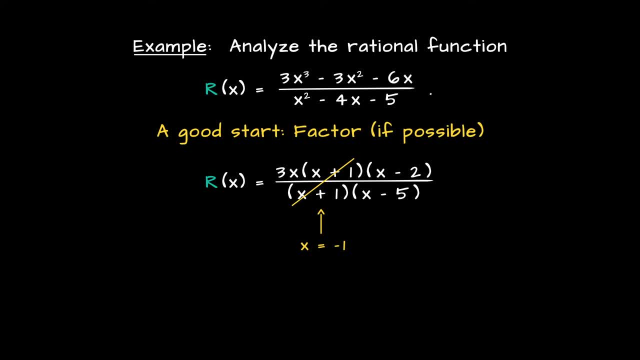 the value of x. that makes the factor equal to 0.. Rather, the rational function will have a removable singularity or whole at x equals negative 1.. It's not defined there because it makes 1 x, 2 x, 0, 0 x x 1. That's the fractional function and the unknown was 0.1, does not join the result. 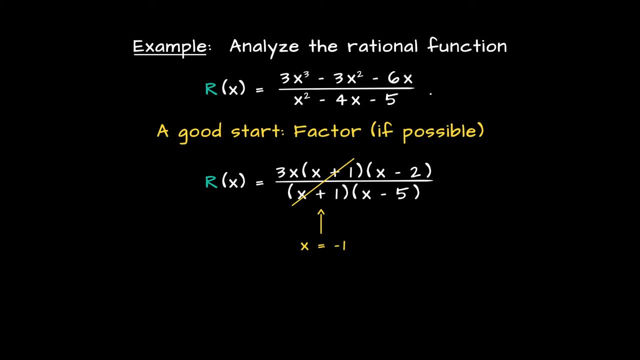 and denominator of the rational function equal to zero, and zero over zero is simply undefined. So this common factor gives us a removal singularity at x equals negative one. As long as x is not equal to negative one, our function takes the form shown here, And since a 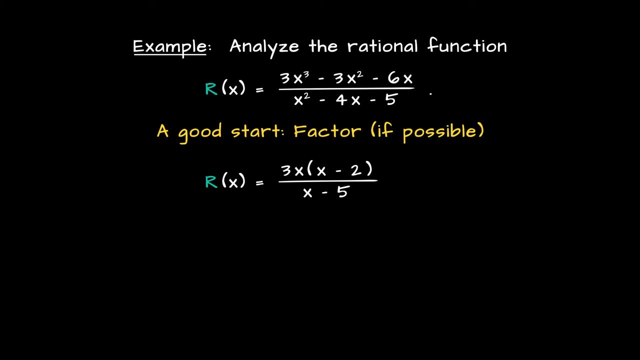 ratio of two things can equal zero only if the numerator is equal to zero. we see that the zeros of this function occur when x is zero and when x is two. On the other hand, this ratio will be undefined when the denominator is equal to zero, and that happens exactly when x is five. That value 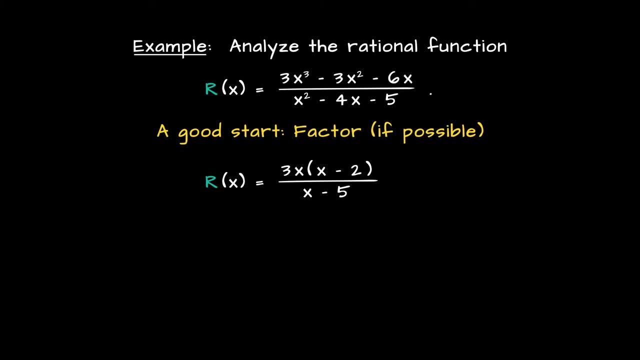 will correspond to a vertical asymptote of our rational function, because if x equals five, the function will, as it were, blow up to infinity. In summary, we saw that this rational function has a removable singularity at x equals negative one, because that's a root of both the numerator and denominator. 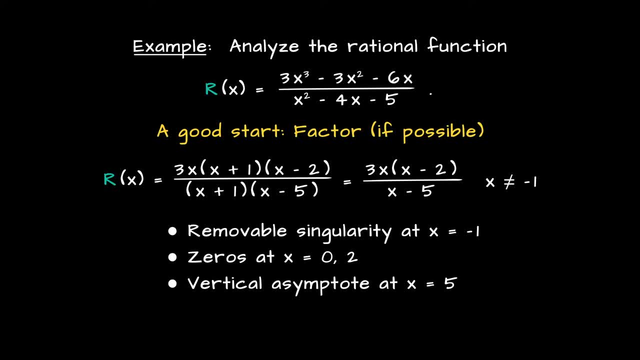 After it's cancelled out, however, our rational function is identical to the function 3x times x minus two, all over x minus five, And that function is equal to zero at zero and two, because that's exactly where the numerator is equal to zero And it has a vertical asymptote. 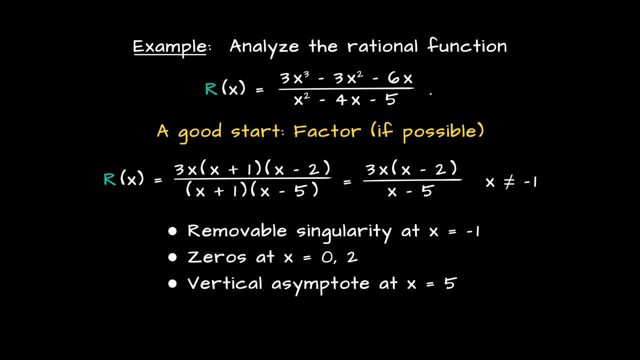 at x equals five, because that's precisely when the denominator is equal to zero. What about the horizontal asymptote of this function? Well, it turns out that there is no horizontal asymptote, and that's because the degree of the numerator of this rational function is greater than the degree of the denominator. 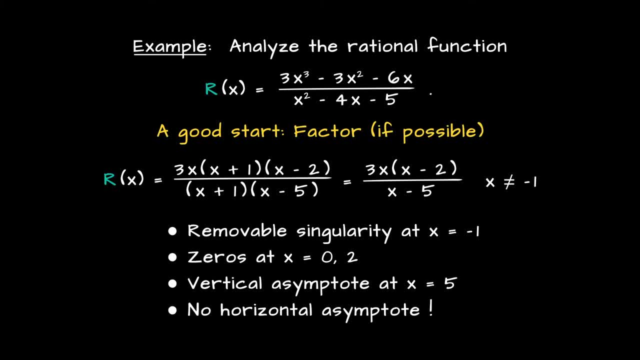 which means that as x goes to positive infinity or to negative infinity, the numerator will rapidly outgrow the denominator and make it impossible for the rational function to approach any constant value. It must in fact go to either positive or negative infinity as x gets large. 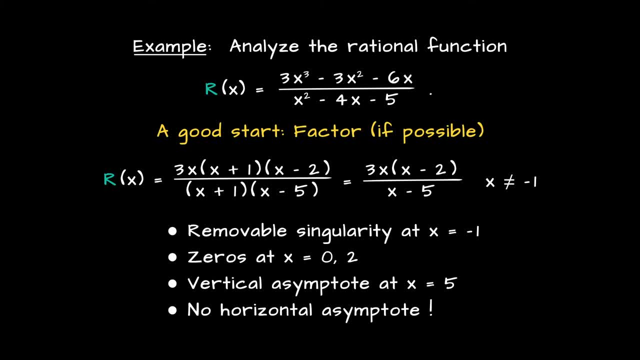 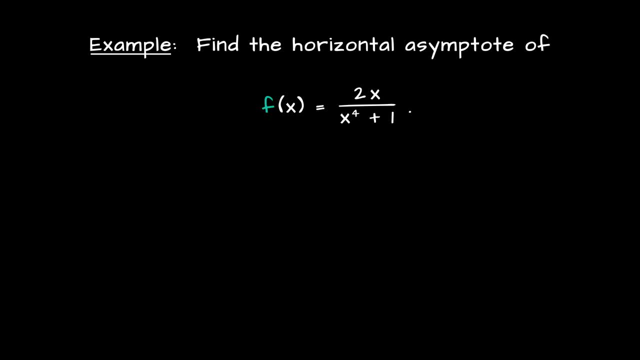 so there will be no horizontal asymptote. Let's try to focus more on horizontal asymptotes by considering a couple quick examples. This first example asks us to think about the horizontal asymptote of the function 2x over x to the fourth plus one. 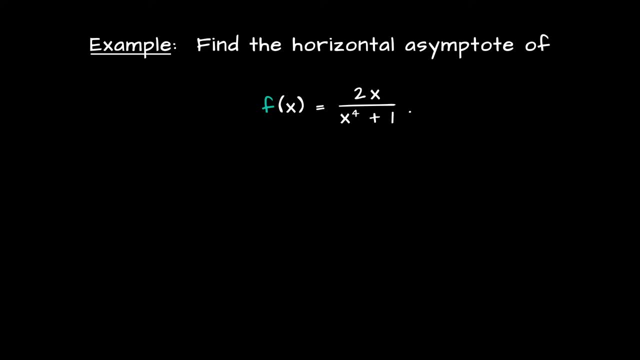 All right. so the question here is what happens to the values of our function as x gets really big in either the positive or the negative directions? And the key thing to realize here is that the numerator is a linear polynomial, whereas the denominator is a polynomial of degree four. 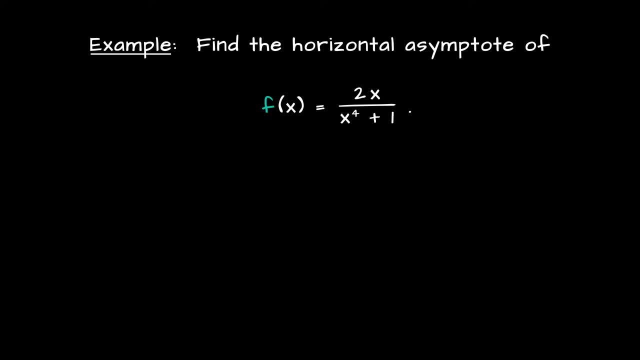 Now, a polynomial of degree four, as we know, grows much more rapidly than a linear polynomial, And so the denominator here will dominate as x gets large. In fact, the values of this function are forced to go to zero for very large values of x. 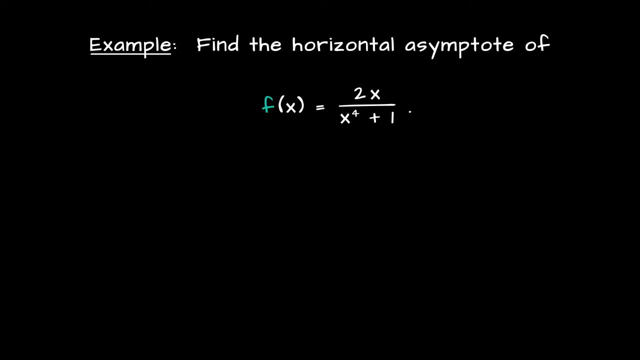 simply because the numerator can't keep up with the growth of the denominator. So the horizontal asymptote here would be the horizontal line. y equals zero. And let's look at one more example. Here's a rational function where the degree of the numerator and the degree of the denominator 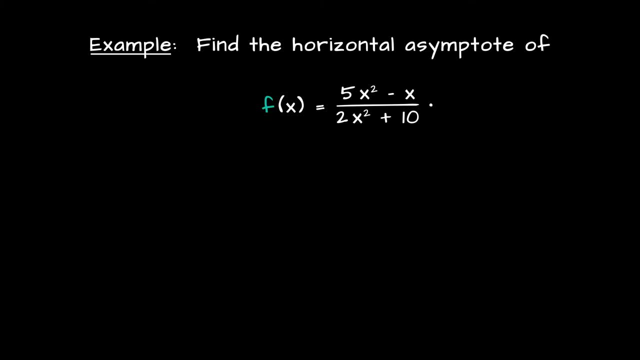 are exactly the same. Let's try to think about what happens with the horizontal asymptote Now. the key idea is that the numerator and denominator should grow at approximately the same rate, And to really understand what's going to happen in the long run when x is large. 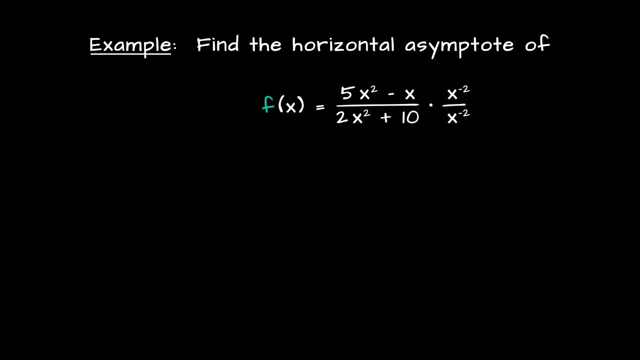 we're going to do the following: We're going to try to multiply this expression by x to the minus two, over x to the minus two. We're choosing minus two here because that matches the degree of the numerator and denominator, And by multiplying by this expression we are not changing the value of our function, right? 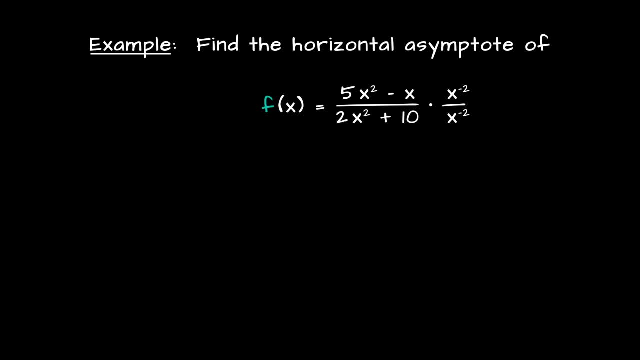 Since it's always equal to one as long as x is non-zero. After we multiply things out, we're left with the following expression, And the key thing to notice here is that, as x gets very large, both the one over x term in the numerator and the 10 over x squared term in the denominator. 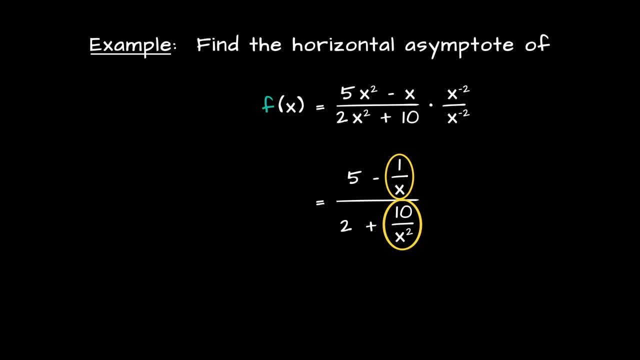 will get closer and closer to zero, And as x gets really large, their values will truly become insignificant, And so the value that f approaches will be less than or equal to zero. And so the value that f approaches will be less than or equal to zero. And so the value that f approaches 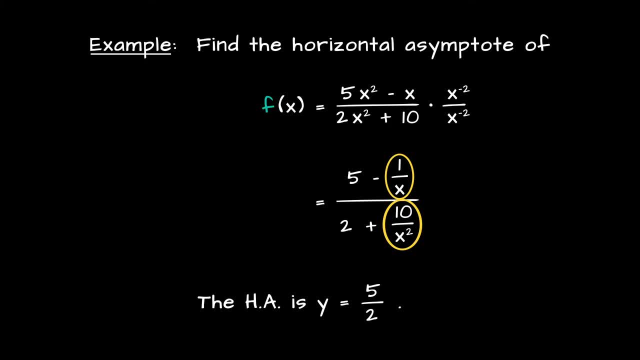 will actually be five over two, And that is nothing other than the ratio of the leading coefficients of the numerator and denominator of the original rational function. So the horizontal asymptote, abbreviated HA, here is: the horizontal line y equals five over two. In summary, the horizontal asymptotes of a rational function.